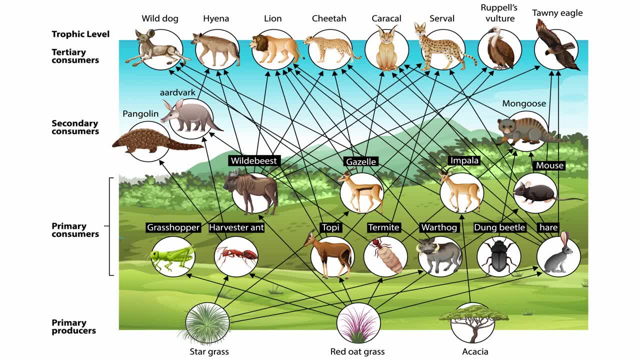 detritivores and then carnivores. Food webs offer an important tool for investigating the ecological interactions that define energy flows and predator-prey relationships. The fundamental purpose of food webs is to describe the feeding relationship among species in a community. All the species in the food webs can be distinguished into basal species. 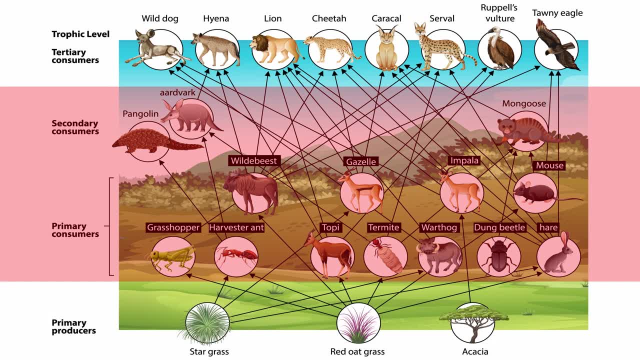 or autotrophs, such as plants, intermediate species like herbivores and intermediate-level carnivores such as grasshoppers and scorpions, or top predators, meaning high-level carnivores such as foxes. These feeding groups are referred to as trophic levels. 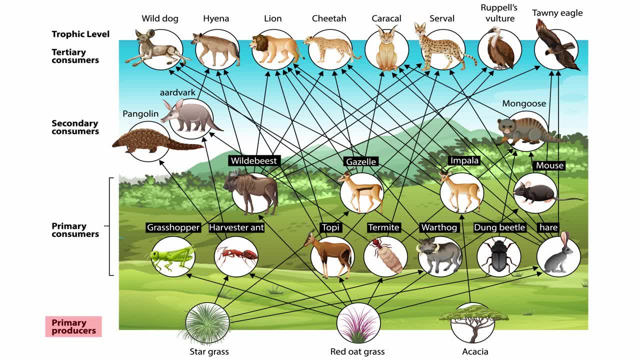 basal species occupy the lowest trophic level. as primary producers, They use solar energy to generate chemical energy and build their own structures. The second trophic level consists of herbivores. These are first consumers. The remaining trophic levels include carnivores. 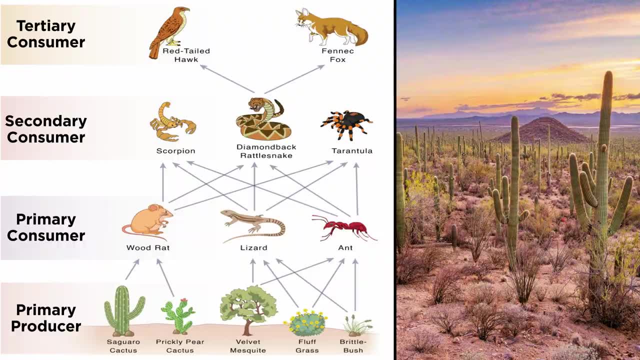 that consume animals at trophic levels below them, For example in a desert environment. the second, consumers located on trophic level three would include birds and scorpions. These animals act as both predator and prey. Continuing tertiary consumers making up. 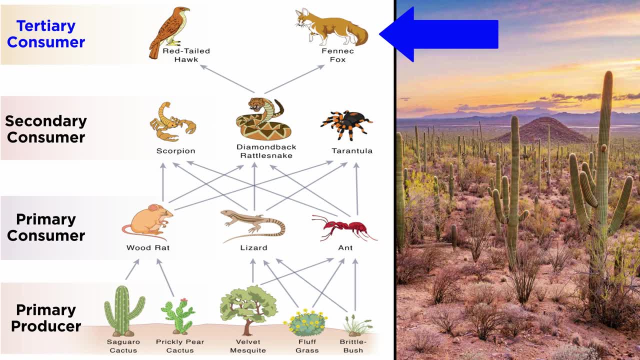 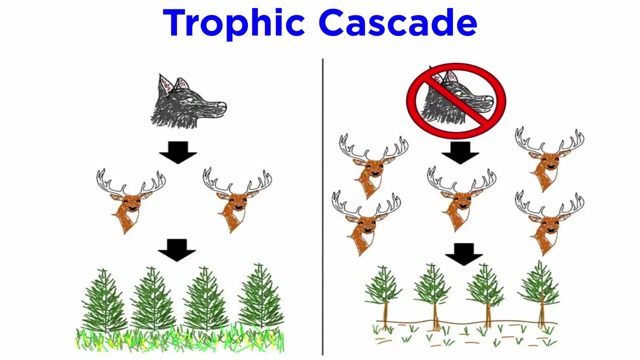 the fourth trophic level include bird predators such as eagles and foxes, or mountain lions. Grouping all species into different functional groups or trophic levels helps us simplify and understand the relationships among these species. Trophic cascades are powerful. 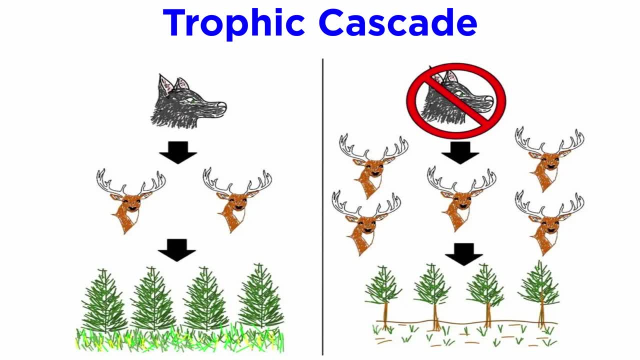 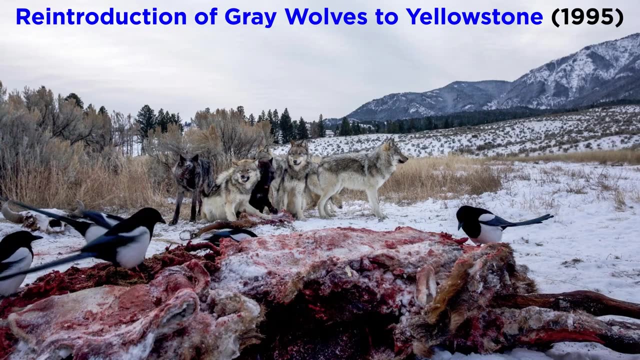 indirect interactions that can control entire ecosystems. These occur when predators limit the density or behavior of their prey and thereby enhance survival of the next lower trophic level. A classic example of such a cascade is the reintroduction of gray wolves to Yellowstone National Park, which reduced the number of elk and changed their behavior Again. 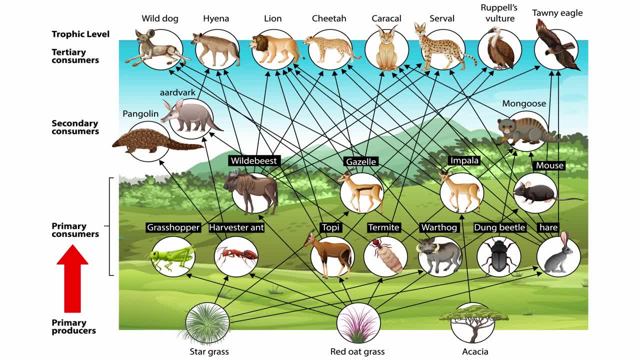 food webs illustrate energy flow from primary producers to primary consumers or herbivores, and from primary consumers to secondary consumers or carnivores. The structure of food webs suggests that productivity and abundance of populations at any given trophic level are controlled by the. 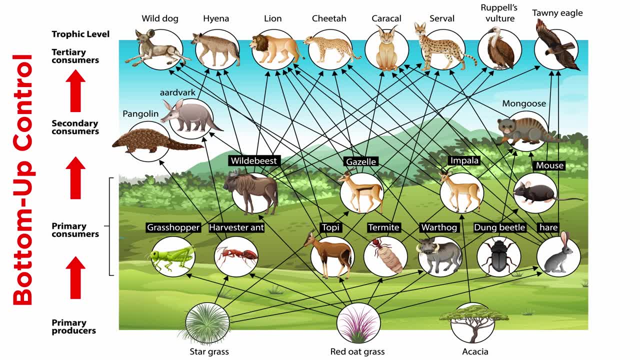 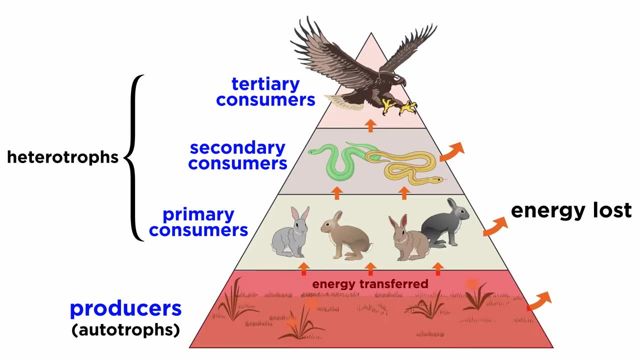 productivity and abundance of populations in the trophic level below them. This phenomenon is called bottom-up control. Correlations in abundance or productivity between consumers and their resources are considered as evidence for bottom-up control. For example, plant population densities control the abundance of herbivore populations, which in turn control the densities. 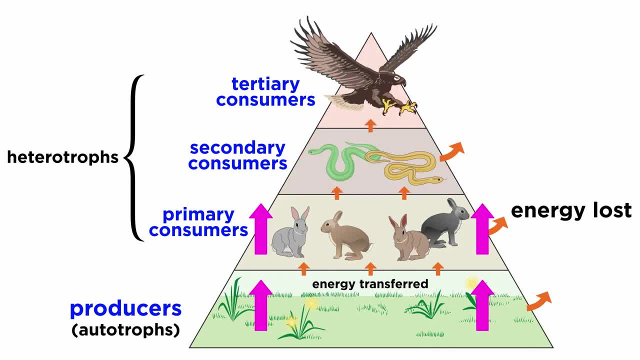 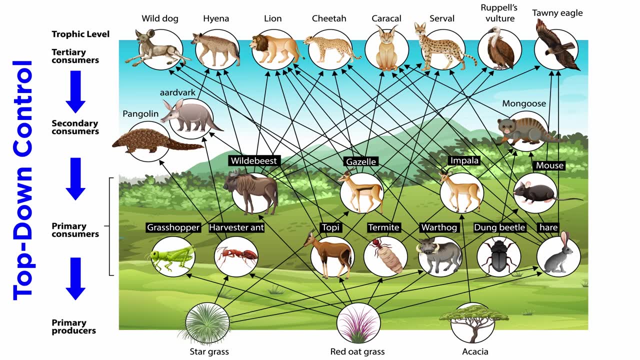 of the carnivores. The same applies to the population density of herbivores. The same applies to herbivore populations. Thus, the biomass of herbivores usually increases with primary productivity in terrestrial ecosystems. Top-down control occurs when the population density of a 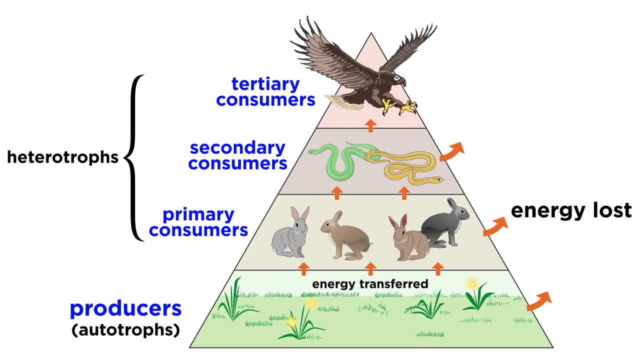 consumer can control that of its resource. For example, predator populations can control the abundance of prey species Under top-down control. the abundance or biomass of lower trophic levels depends on effects from consumers at higher trophic levels. A trophic cascade is a type of 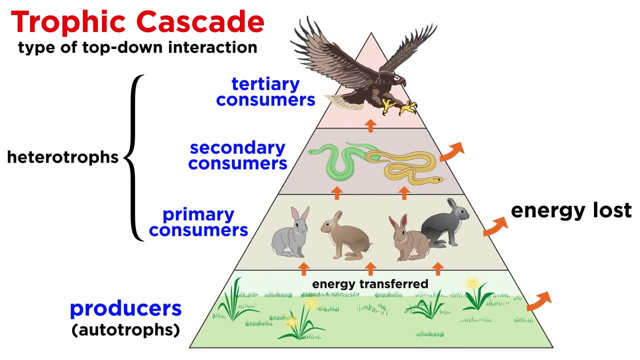 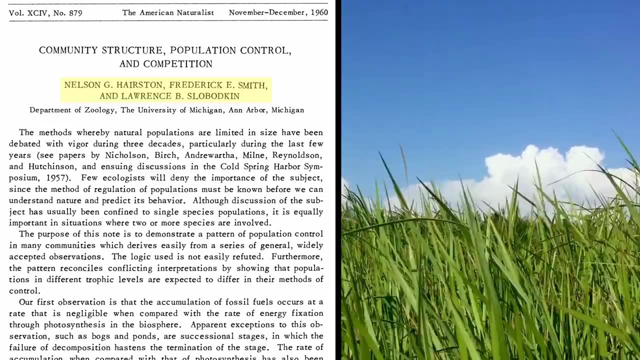 top-down interaction that describes the indirect effects of predators In a trophic cascade. predators induce effects that cascade down the food chain and affect biomass of organisms at least two lengths away. Nelson Hairston, Frederick Smith and Larry Slobodkin first introduced the 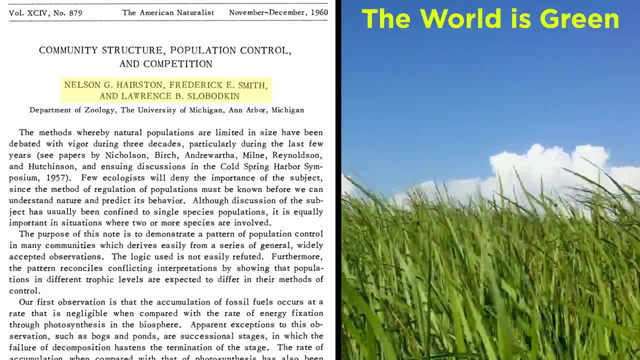 concept of top-down control with the frequently quoted the world is green proposition. They proposed that the world is green because carnivores depress herbivores and that the world is green. The concept of top-down control is that the world is green because carnivores depress herbivores. 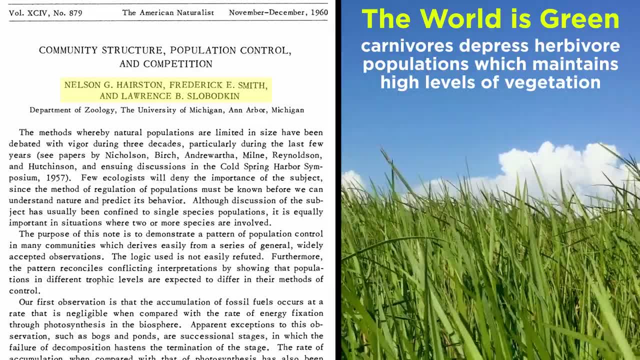 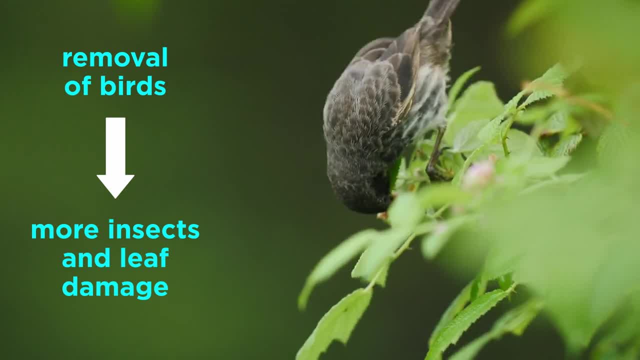 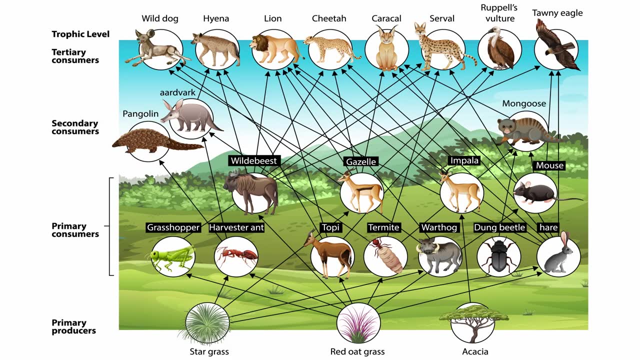 and keep herbivore populations in check. Otherwise, herbivores would consume most of the vegetation. Indeed, a bird exclusion study demonstrated that there were significantly more insects and leaf damage in plots without birds compared to the control. Now that we've covered food webs and trophic cascades, we are beginning to understand how. 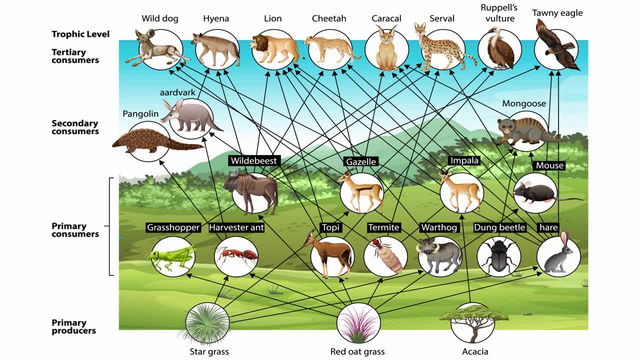 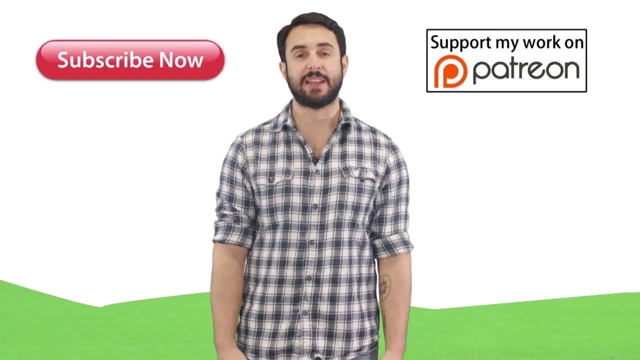 interactions between species in a community have profound effects on an ecosystem as a whole. Let's continue this line of thought. If you're interested in learning more about herbivores, please subscribe to our channel and, as always, feel free to email me. 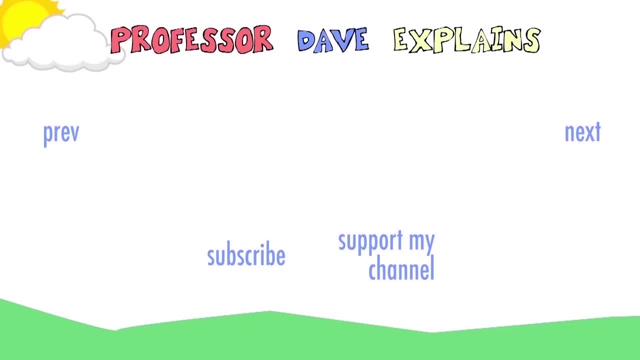 Thank you for watching and I'll see you in the next video.